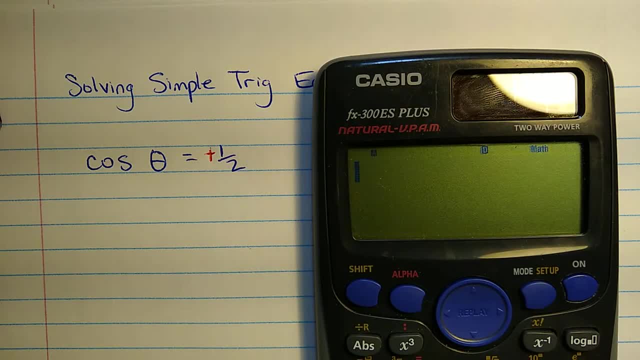 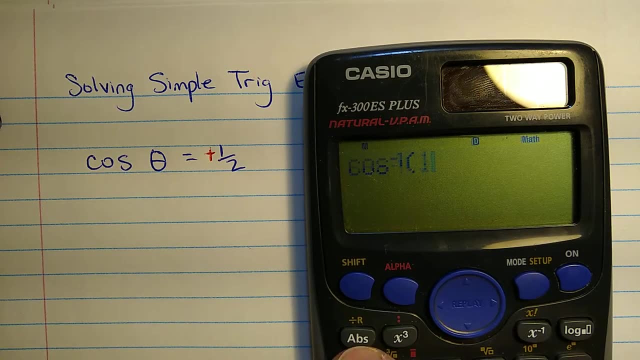 I'm just going to use a calculator to show you how that part works. So what we'll do is we'll use the cosine inverse function on the calculator and we'll put in one half. You can put in the fraction, or you can put in the number 0.5, and I get 60.. 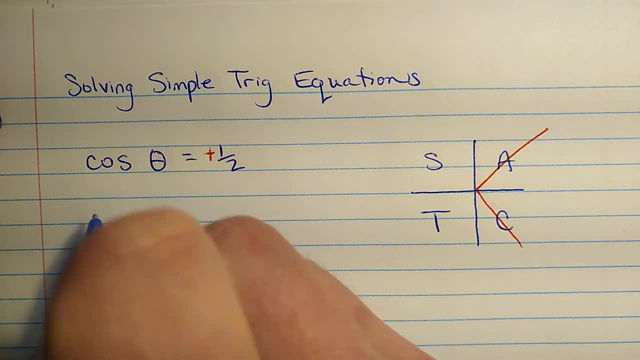 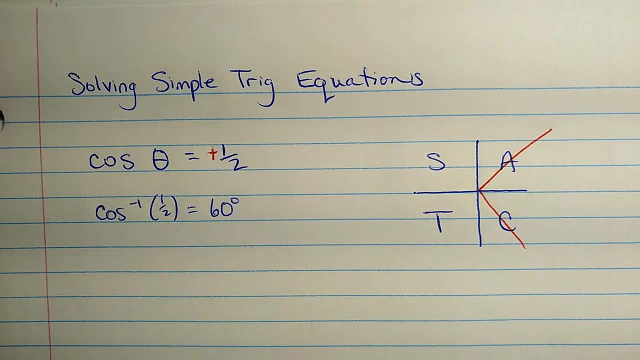 And this is in degrees right now, so 60 degrees. I'm just going to write it like this, Notice: I'm not going to write theta equals, so I'll just write: cosine inverse of one half is 60 degrees. Now, that is the quadrant one solution, but there's another corresponding quadrant two solution. 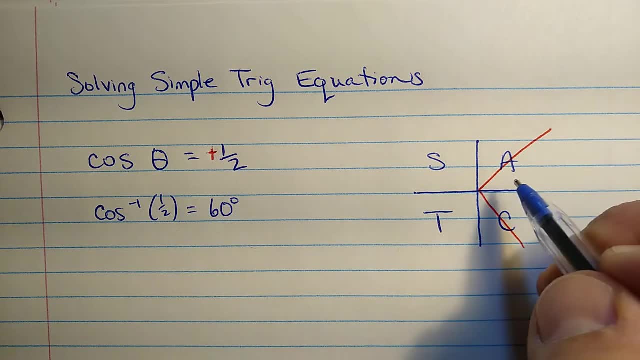 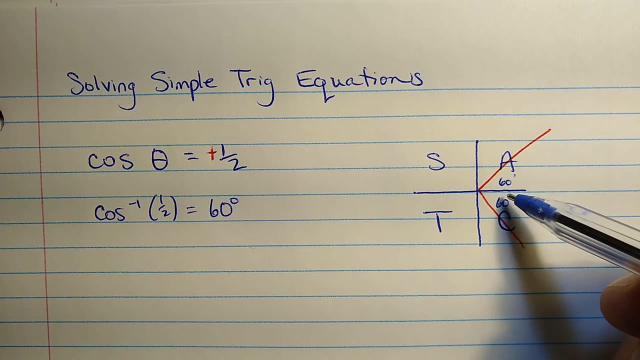 Okay. so first off, let's notice this is an acute angle. It would be the acute angle right here, 60 degrees. And so there's another related angle with the same cosine, which is 60 degrees from the x-axis, this direction. 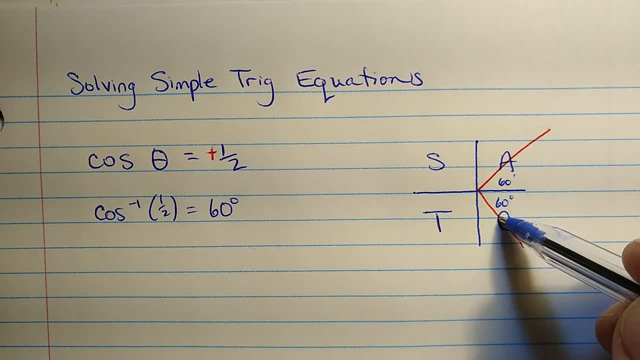 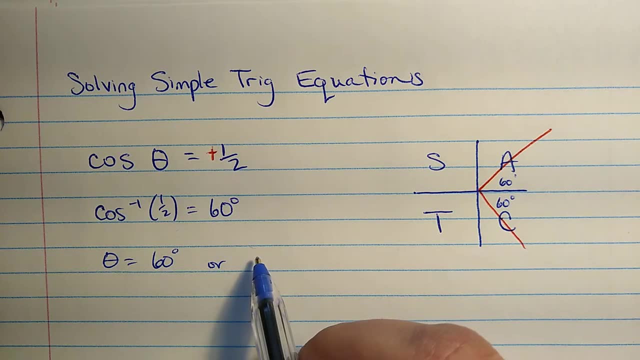 That is 360 minus 60.. So one of our solutions is 60 degrees and the other solution is 360 minus 60, or 300 degrees. Let me just write that down how I got that: That was 360 degrees. 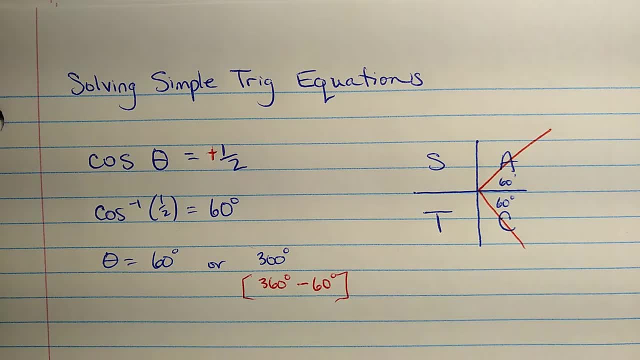 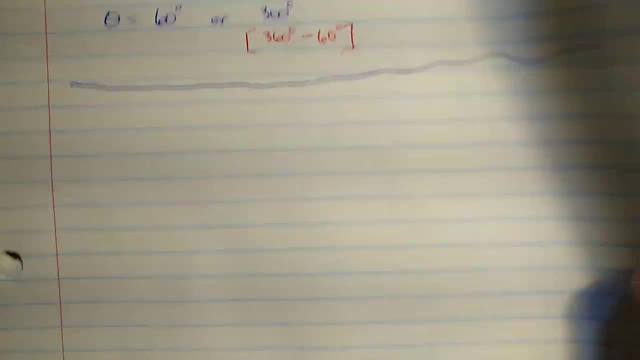 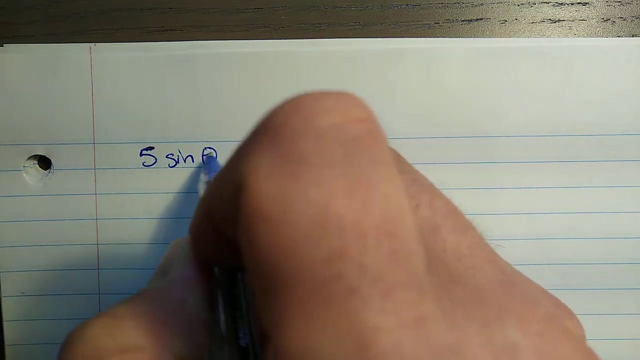 minus the acute angle, 60. That's where that came from. So those are the two solutions to this equation. All right, let's do one that's a little more complicated Fresh page. How about this? one? Five times the sine of theta plus one equals negative two. 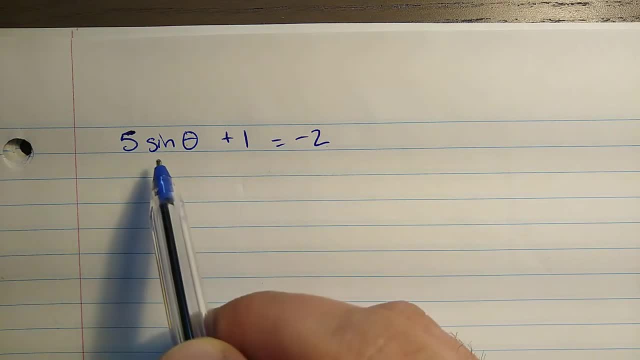 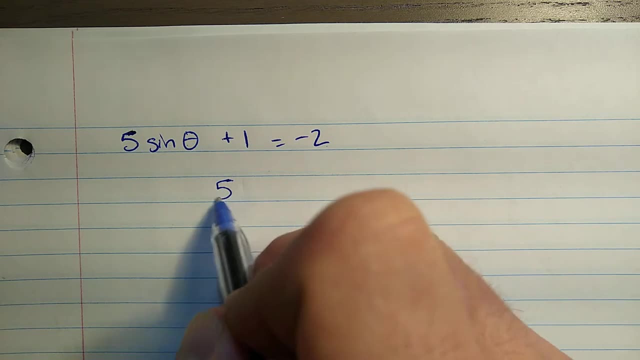 Now this one's only more complicated because it has some extra terms in it. Notice we still have just sine theta here. That's pretty doable. I'm going to subtract one from both sides. I'll have five. sine theta equals negative two minus one is negative three. 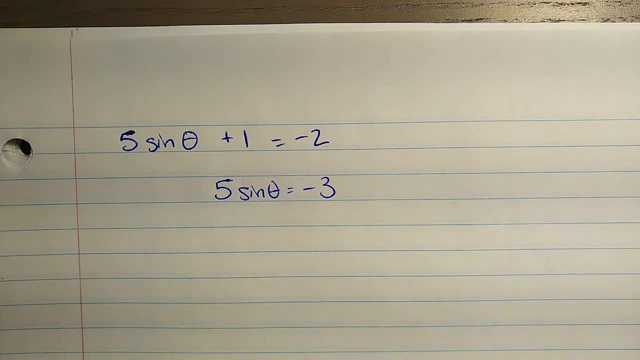 Now, sine of theta is one piece, It's a function, sort of like f of x, And so I can just divide both sides of this equation by five, and I'll be left with sine theta on the left-hand side, on its own. 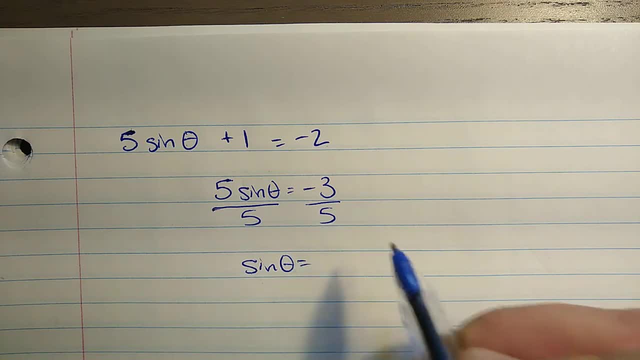 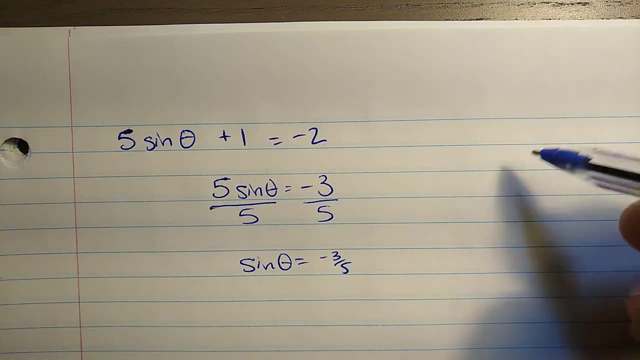 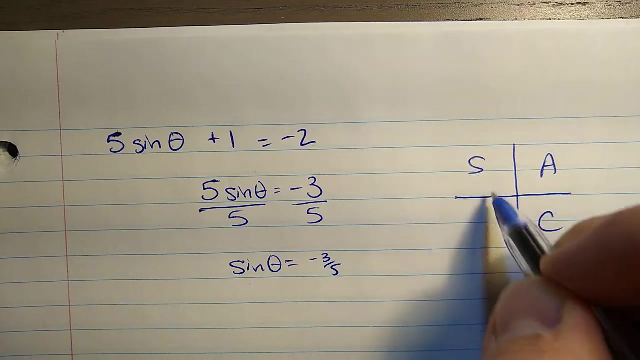 This is five times sine theta divided by five, And I have this equation Now. notice how similar that is to what we worked with in the last example. Primary trig ratio equals a number Cast rule, And I recommend just draw this out for yourself as you work. 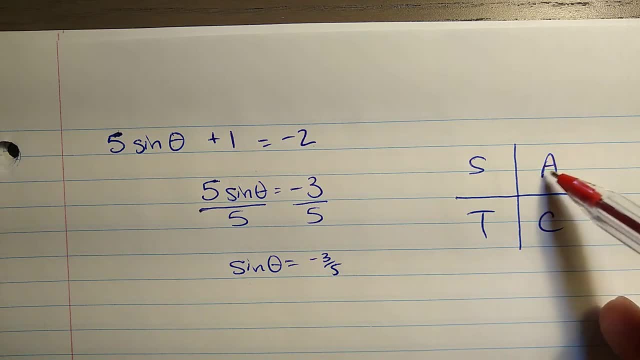 Sine has to be a negative number. Sine is everything's positive here. Sine is positive there. That means I'm going to have something there and something there. Grab my calculator. Sine of theta is negative three-fifths. 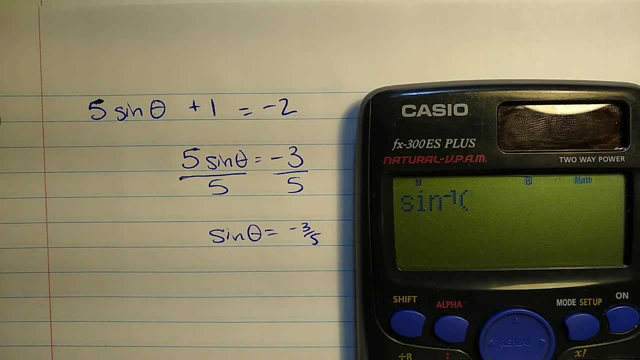 So let's do sine inverse. So in my calculator shift and then just above the sine button Negative three-fifths. Again, you can use a fraction if you want, Or in that case you can put negative 0.6.. 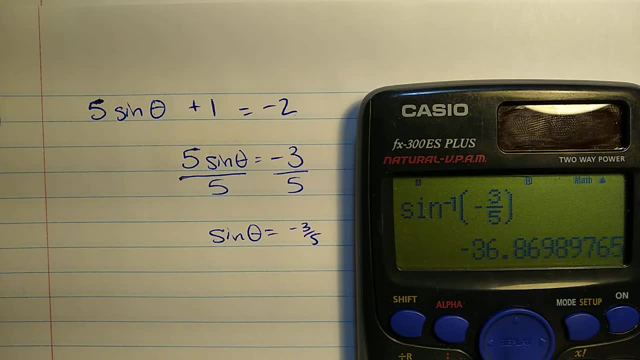 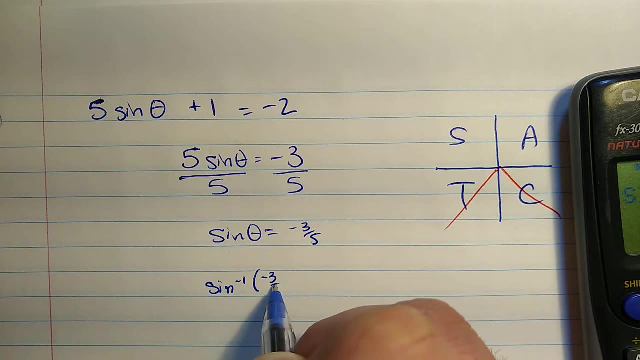 And I get, oh, not such a nice number, In fact a negative number. Let me write this down just like I see it on my calculator: Sine inverse of negative three-fifths is about negative 30.. Well, we'll just write negative 37.. 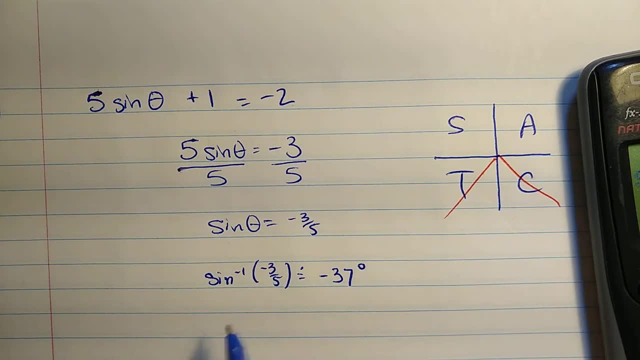 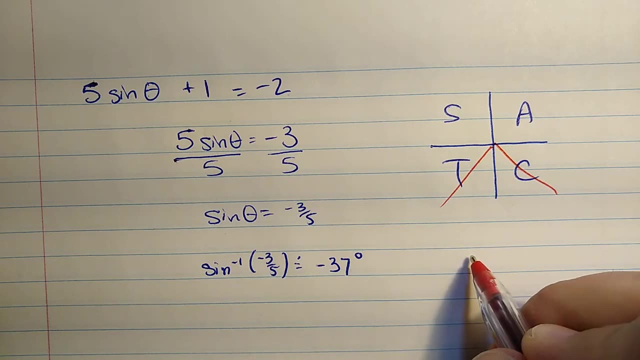 We'll round off Now. here's the thing about the inverse functions. on your calculator They give you angles that are between negative 180 and positive 180. Those are the angles that they give. Maybe they give exactly 180. I can't remember now. 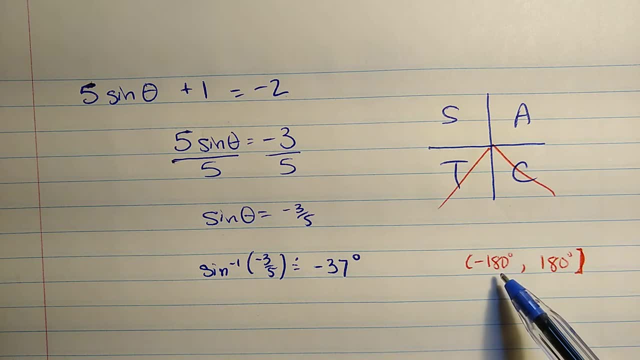 They don't give you angles like 200 degrees, They only give you angles between negative 180 and positive 180.. And so what this means? the negative ones are counted from the positive x-axis going clockwise. So, for example, this red line that I drew here looks like about negative 45 degrees. 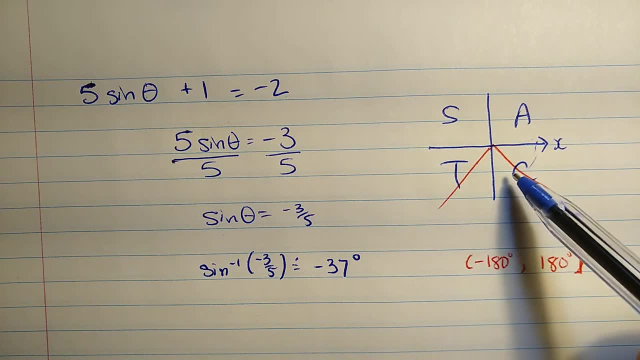 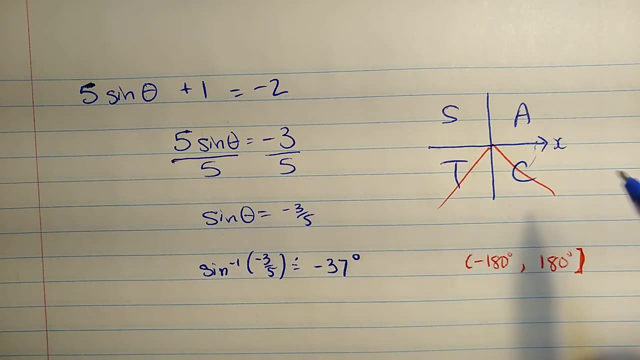 That's how your calculator would say it. It would not go all the way around and say 315 degrees. So the negative ones are down here. The positive ones are here counting from the x-axis. So negative 37 is 37 degrees clockwise from the x-axis.